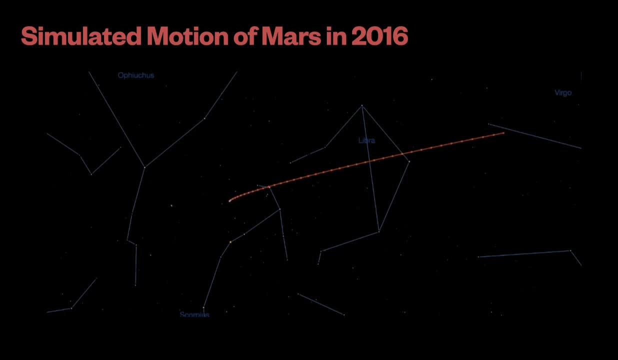 Along the sky. it slows its position and then reverses its direction. We'll see. it reverses its direction again and then keeps on going. So just from this data, or these observations alone, it certainly isn't clear that Mars is an elliptical orbit around the sun. 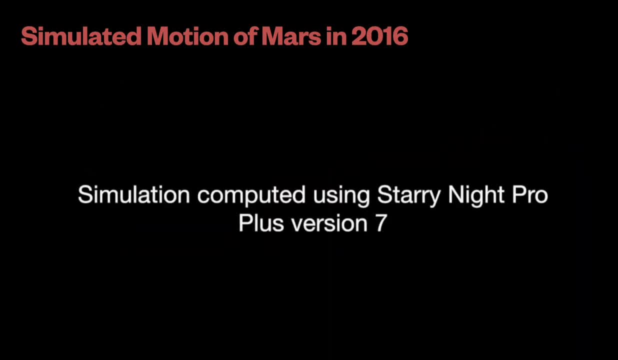 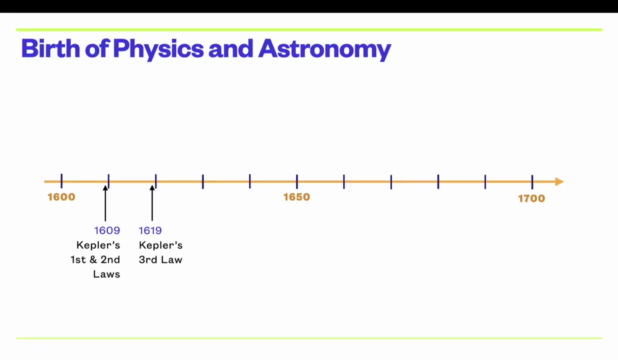 But by making very precise model calculations of different planet possible planetary orbits, Kepler showed that the only way of explaining that motion of Mars against the background stars was if it followed an elliptical orbit. So Kepler developed three laws of motion, the first of which says that the planets orbit in elliptical orbits in 1609.. 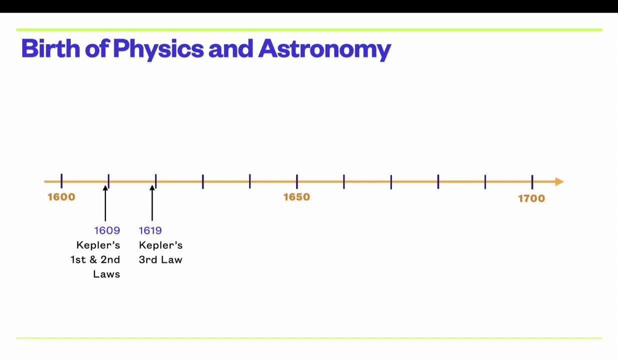 1609.. So Kepler had known this for at least eight years before he came to a conclusion. This was a year before the invention of the telescope and Galileo's first observations of the night sky with a telescope. So again, this preceded telescopic observations, which is pretty amazing. 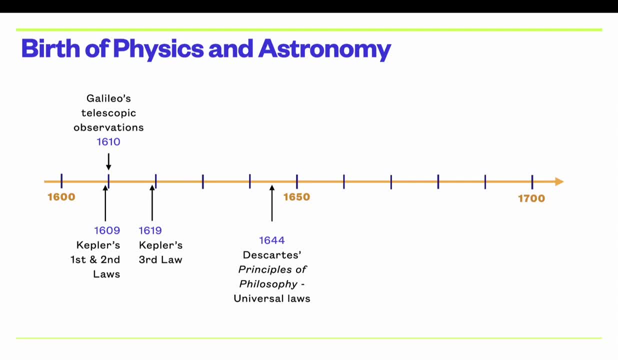 Just for historical context, It's also interesting to think that That Newton's idea that Kepler's firm heart went in the same direction that Kepler's base idea. it's pretty beautiful, очень proud was coming up with this idea that they're. 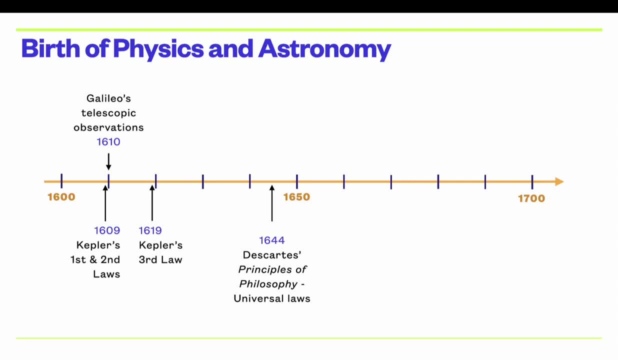 That the universe is governed by a universal set of physical laws, Universal laws and forces. Those ideas weren't forming until a good you know thirty or forty years after Kepler's observations. It wasn't until much later, in the late sixteen hundreds, that Newton took Kepler's discovery that planets orbit the Sun in a possono different way. 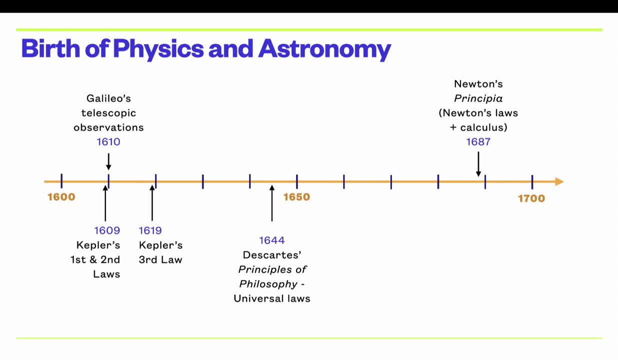 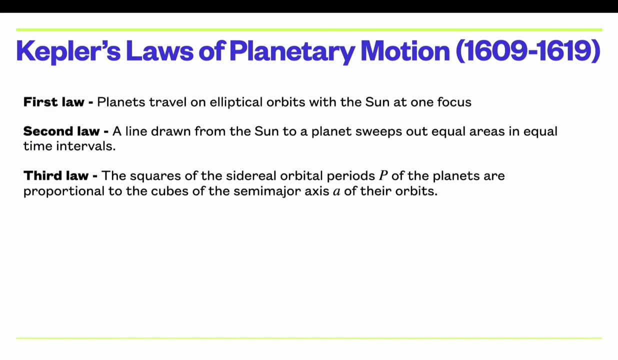 It isn't that simple: elliptical orbits, and from that observation deduced newton's now famous three laws of motion. so f equals m, a was actually an invention used to describe kepler's observations. so in this lecture we're going to define kepler's three laws. 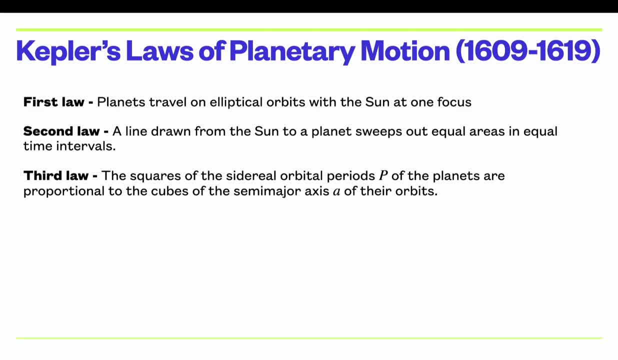 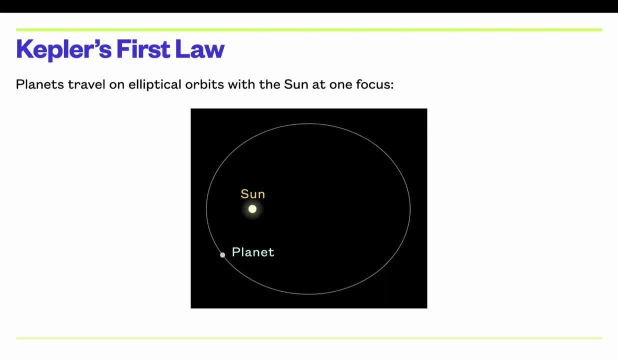 um, and then in subsequent lectures we'll talk about how to derive those laws from newtonian mechanics. kepler's first law says that planets travel in elliptical orbits with the sun at one focus. so here's a sketch of an elliptical orbit with a planet on it. the sun is at one focus. 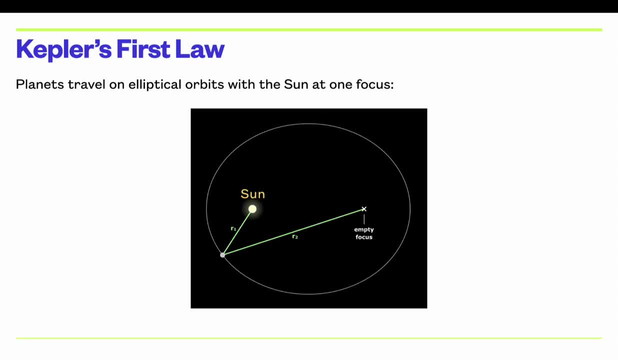 at the other focus is just empty space. so let's define a few properties of an ellipse. uh, let's put a little plus sign at the center of the ellipse. the distance from the center out to the long edge of the ellipse is called the semi-major axis. it's usually given by the letter a. 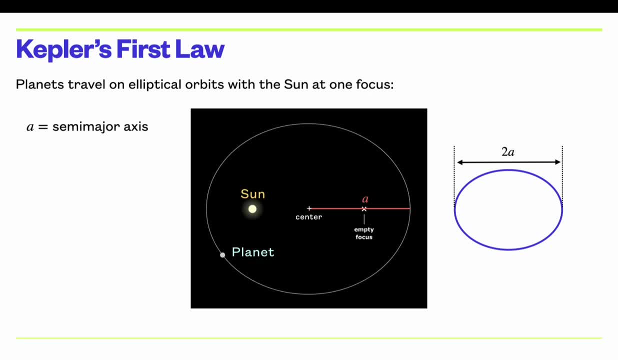 if you look at the, the complete diameter or distance across the ellipse, that would be two, and then you can see that the center of the ellipse is the center of the ellipse. so if you look at the center of the ellipse, you can see that the center of the ellipse is the. 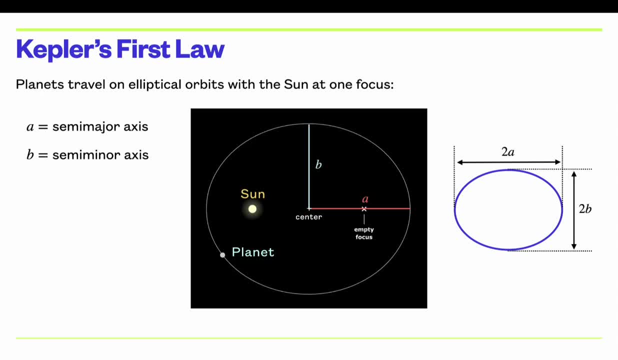 short side of the ellipse is called the semi-minor axis b, and so the total distance across the short, the short width of the ellipse, is uh, 2b, uh, and then the eccentricity, e. uh is a measure of like how squashed the ellipses. so it's defined. 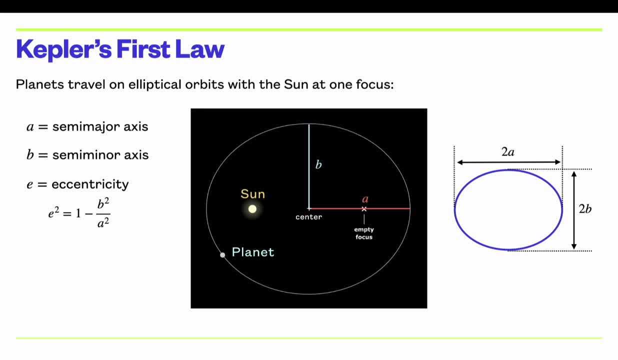 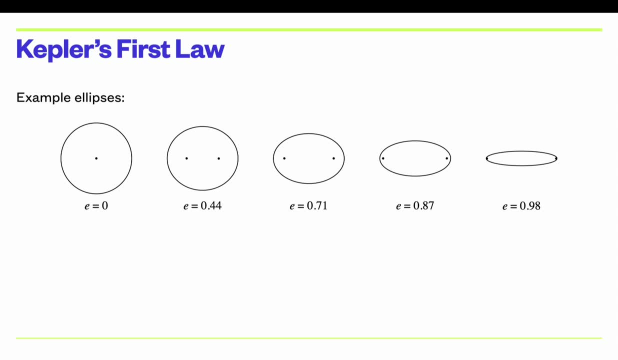 as e squared, that is, the eccentricity squared, is 1 minus b squared over a squared. so here are some examples. so an ellipse with an eccentricity 0 is just a perfect circle. as the eccentricity increases to 1, the the ellipse gets more and more flattened out. 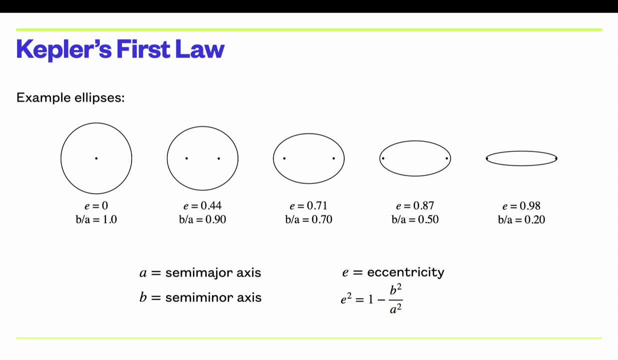 so again, remember that the eccentricity is 1 minus b squared over a squared. so if in a perfect circle b equals a, if b equals a, here you get 1 minus 1 and then you just get 0.. as b gets smaller and smaller, as it gets more squished. 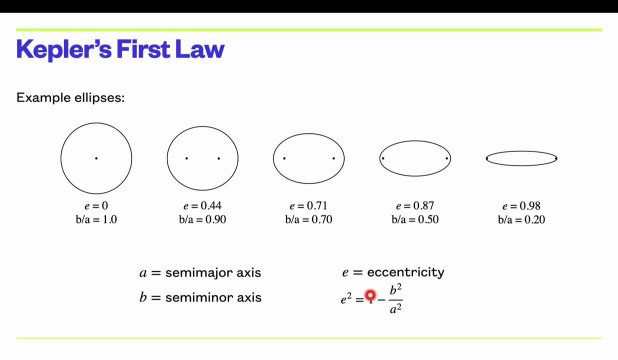 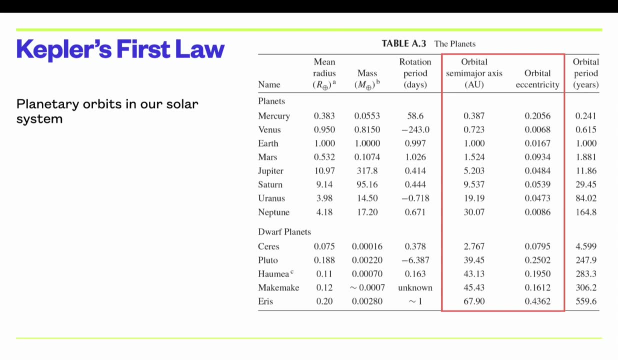 this goes to zero. this term goes to zero, and then e squared just equals one. let's look at the eccentricities of planets in our solar system. so this table is in the back of the of your textbook, it's in appendix a, so the planets mercury, through neptune are listed back there, and 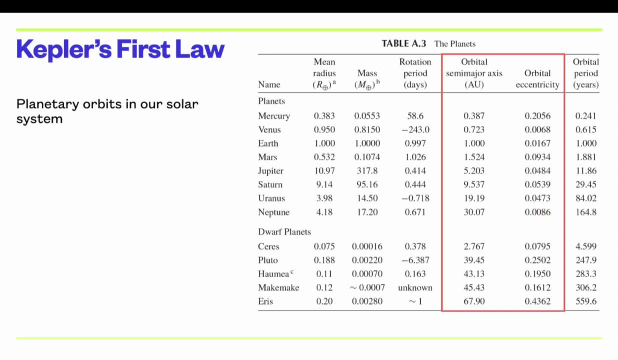 their orbital eccentricities are given in this column. so um. so the earth has a very small eccentricity, 0.016, so it's very nearly a nice circular orbit. mercury is the most eccentric, having an eccentricity of 0.2, so it's the most squashed. uh, your book also lists, uh, the dwarf. 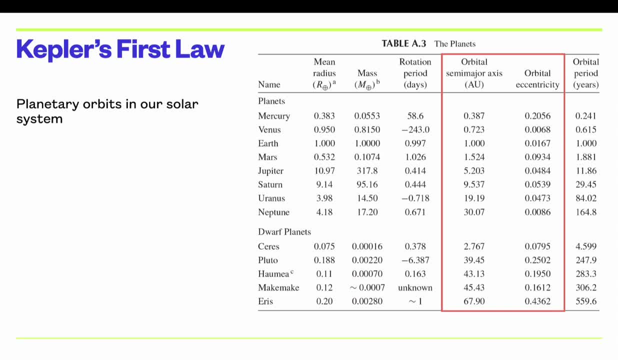 planet. so if you remember, a few years back, pluto was demoted being a dwarf planet. and then there are these other series, humeya, makimaki and harris um, and you can see their properties. this table also includes the uh semi-major axis of the different uh planets in units of astronomical 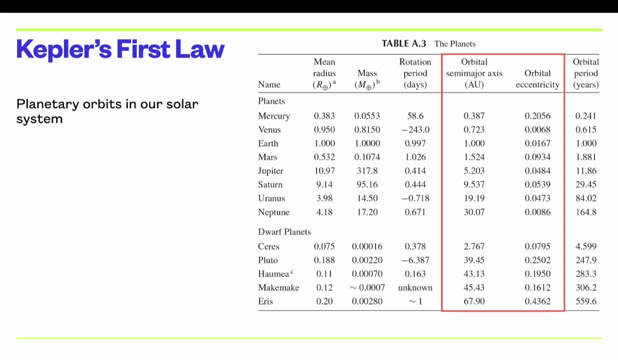 units, which is the average distance from the earth to the sun. so by definition, the earth is. the semi-major axis of the earth is one, and so you can see mercury is about a third of that, neptune is about 30 times that, and a lot of these dwarf planets are even farther out in the solar 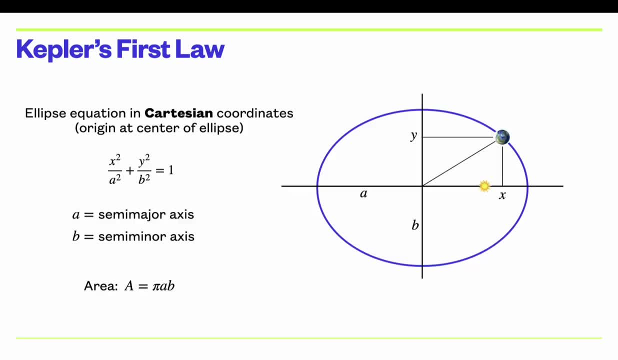 system. okay, so let's write down the mathematical form of an ellipse and a couple of different ways. uh, if we use cartesian coordinates, so if you measure the x and y coordinates of a planet as it goes around um the center, you could define ellipse this way: x squared over a squared, plus y squared, b squared, equals one. remember again, a is a semi-major axis. 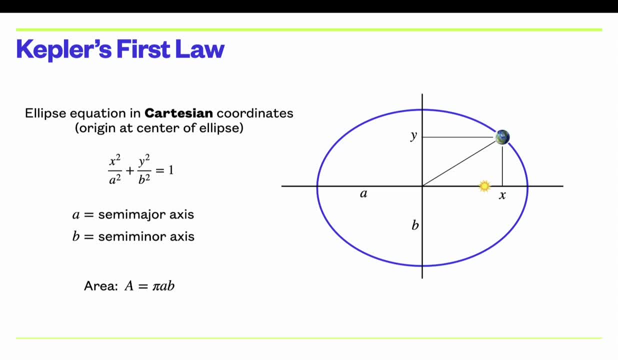 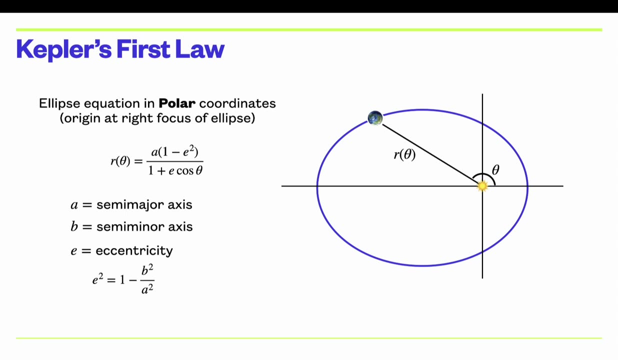 b is a semi-minor axis, it turns out this is not a particularly useful way of describing an ellipse, even though it might be the one that you're most familiar with. A more useful description is to use polar coordinates. So in the previous example the center of the ellipse was at the origin. 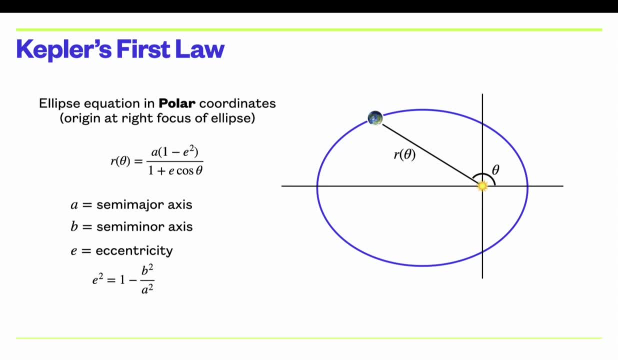 When we write the path of an ellipse in polar coordinates, it's most convenient to place one focus at the origin. So we've shifted the ellipse over. We're going to place the sun, say, at the origin, and then this equation will describe the distance the planet is from the sun. 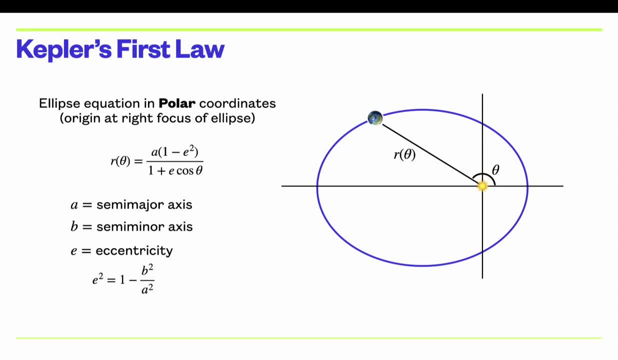 as a function of theta, that is, as a function of the angle as the planet orbits around the sun. So you can see that this expression depends on the eccentricity and the semi-major axis And, of course, on that angle, theta. 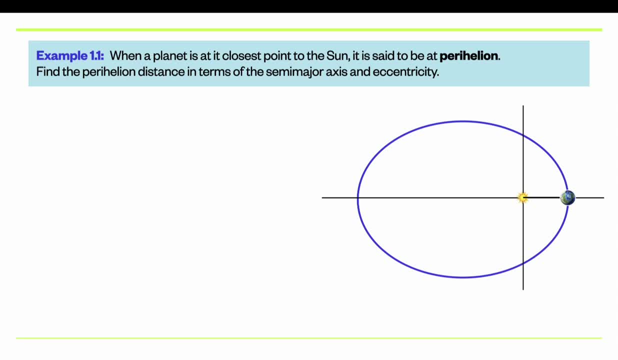 So here's an example: Let's calculate the distance the planet is from the sun at its closest point. So this closest approach is called perihelion, And so we want to find that distance based on the previous formula. So in polar coordinates the perihelion occurs when that angle theta is equal to zero degrees. 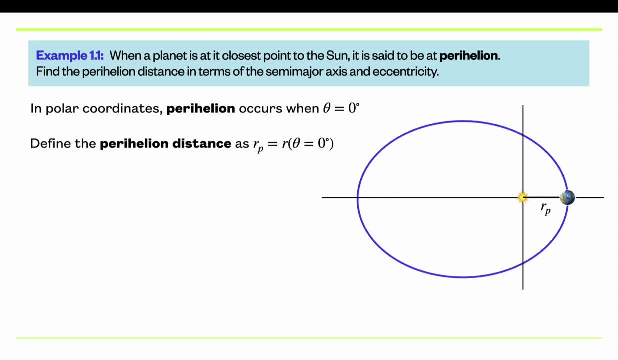 by definition. So we'll define that distance as rp Again. p for perihelion r is the radial distance of the planet to the sun, And so the perihelion distance is that radial coordinate evaluated at theta equals zero degrees. 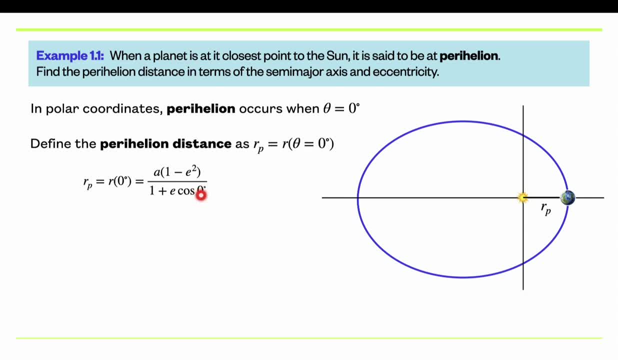 So all we have to do is plug in theta equals zero into our formula here to get the result. Cosine of theta is just one, So we get a times one minus e squared over just one plus e. We can simplify this fraction by expanding the top One minus e squared is just one minus e. 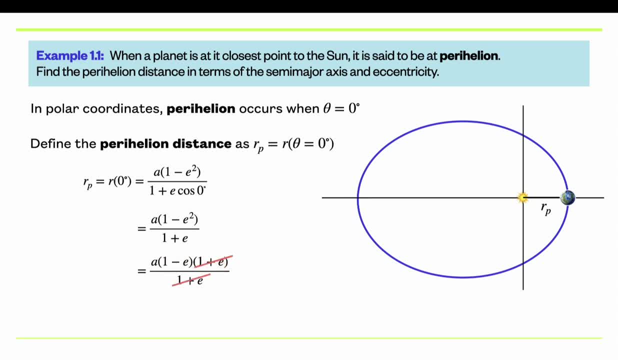 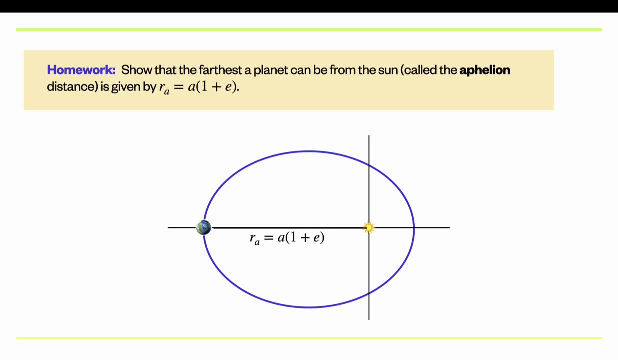 times one plus e. The one plus e's cancel out And we get a very simple result: that the perihelion distance is the semi-major axis times one minus the eccentricity. So as a homework problem, you want to show that the farthest a planet can get from the sun. 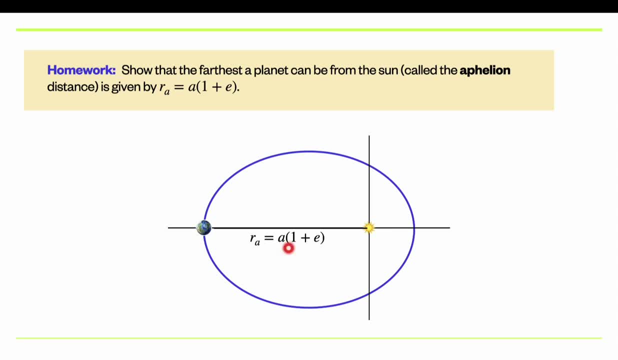 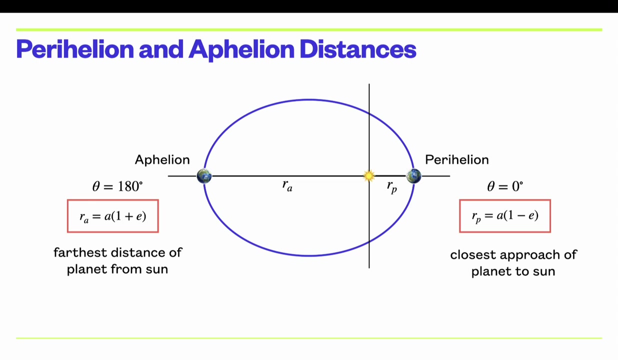 is the semi-major axis times one plus e instead of one minus e. So it's just following the previous formula calculation on the previous slide. but now you want to evaluate it at an angle theta of 180 degrees instead of zero degrees. So here's again just a summary. 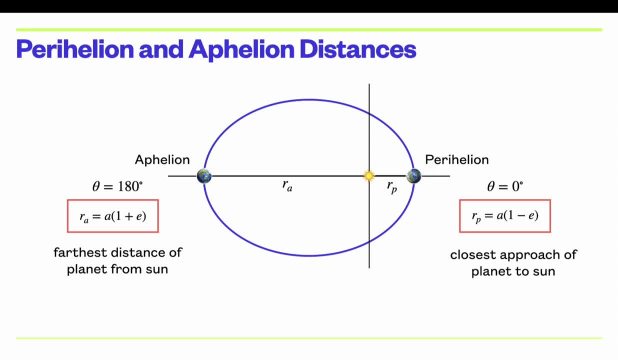 Again, the point of closest approach is called perihelion. That distance is given by a times 1 minus e. The point where the planet is farthest from the Sun is called aphelion, and that's a times 1 plus e. These expressions we'll use over 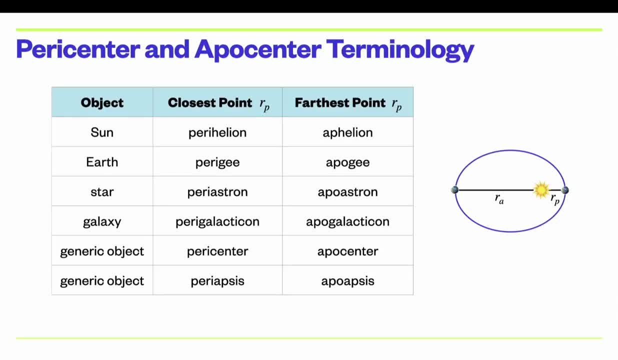 and over in this unit. So it's kind of interesting. Those points of closest approach and farthest approach are called perihelion and aphelion. if an object is orbiting the Sun, If an object is orbiting the Earth, you call those. 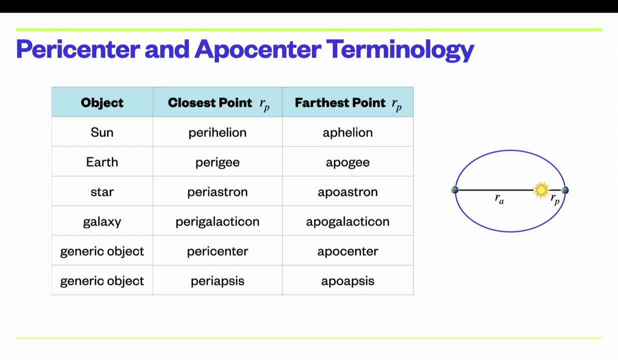 perigee and apogee. If it's orbiting another star, like an exoplanet is orbiting a different star. it's called periastron and apoastron If you've got a star orbiting a galaxy. 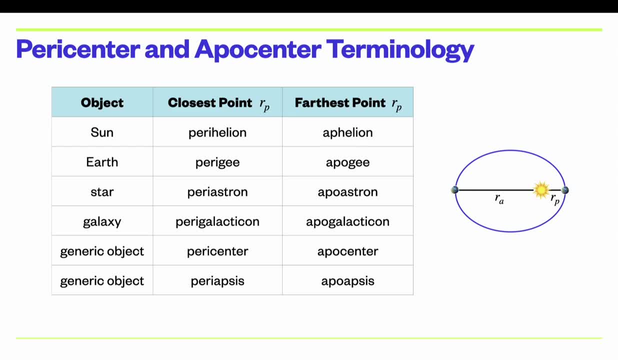 such as our solar systems going around the center of our galaxy. when we're closest to the center of the galaxy, that's called perigalacticon, and when we are farthest, it's called apogalacticon. Your book uses a more kind of generic. 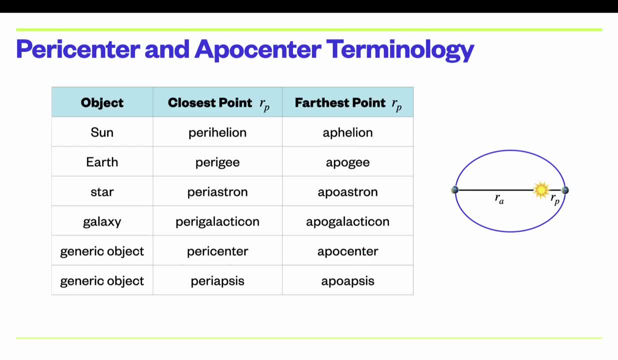 term. They use the term pericenter and apocenter. That just is a generic name, for it doesn't matter what object you're going around, you can call it that. Another term is periapsis and apoapsis. Anyway, there's a million different names. 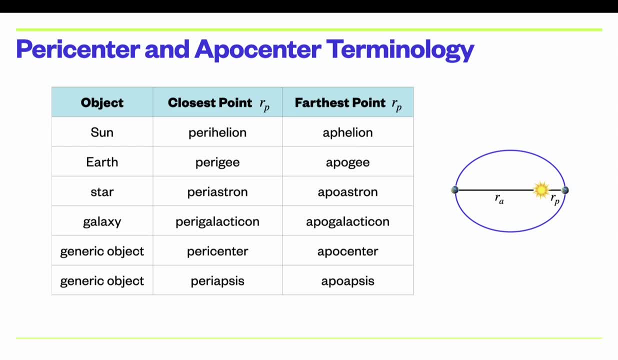 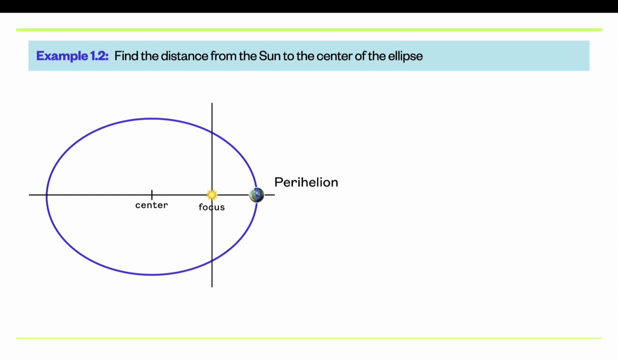 for these points In our solar system. we'll be using perihelion and aphelion, but just be aware that this other terminology is out there. Okay, let's do a another quick example. Let's try to find the distance of the Sun or one of the 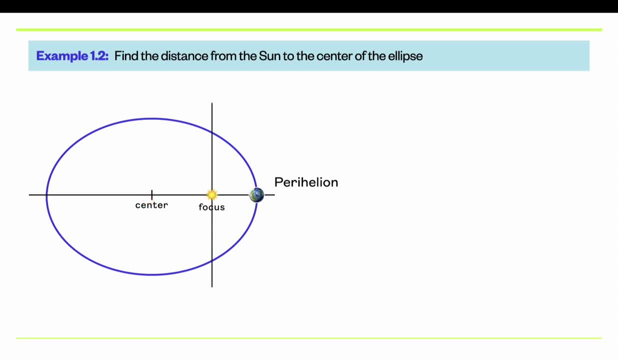 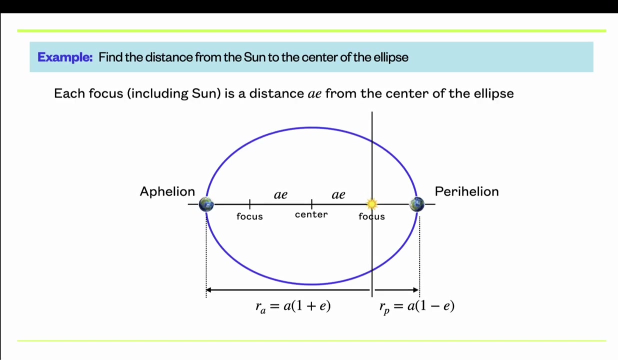 foci to the center of the ellipse. So this is pretty simple calculation given our previous result. That distance from the center out to the focus is just a times e. Very simple result Here. this diagram shows kind of everything we've derived so far. It's got. 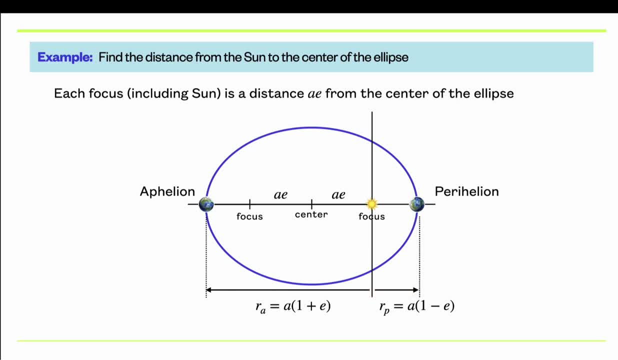 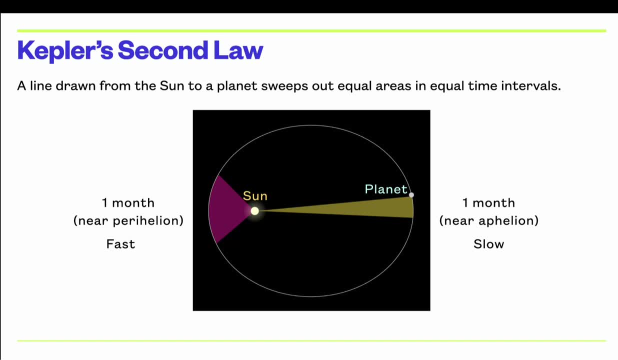 the perihelion distance, the aphelion distance and then how far the foci out are out from the center of the ellipse. Okay, so that gives a few mathematical results about defining an ellipse so that we can describe that elliptical. 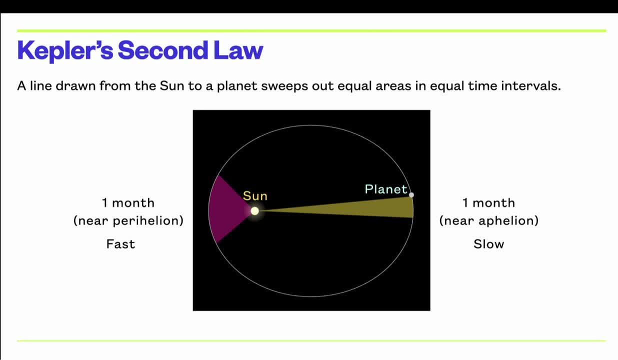 path of a planet around the Sun. Kepler's second law says that a line drawn from the Sun to a planet sweeps out equal areas at equal time intervals. So what that means is that, basically, the velocity of a planet changes as it swings around its elliptical orbit, and 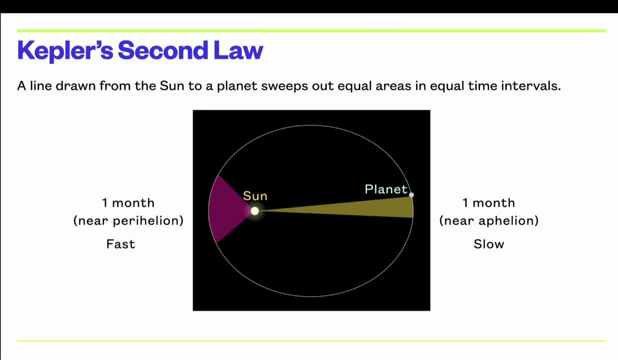 the way that it changes its speed follows this law. So if you've got a planet that's near aphelion- the farthest it is from the Sun, and you've got a planet that's near aphelion- the farthest it is from the Sun, and you let the planet 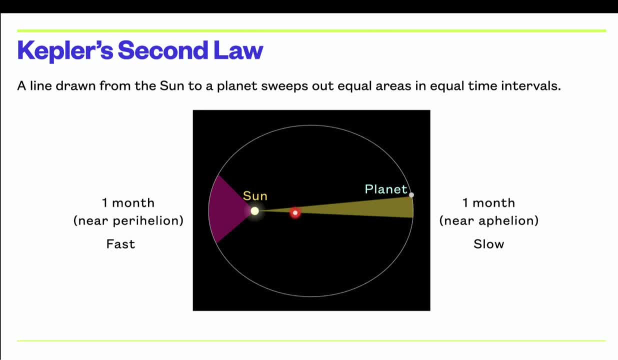 go for, say, a month and you see how far it goes. then the planet will kind of trace out this kind of pie-shaped shape When it comes in and swings closer to the Sun. the area after one month here is going to be the same as the area here, because the planet is now. 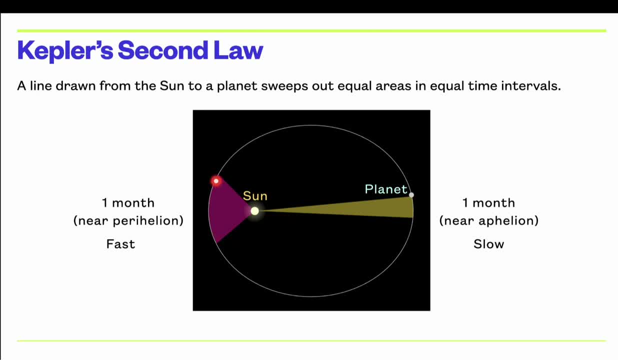 closer to the Sun, it's got to move faster to trace out a farther distance along the arc to have this area match that area. So that means it's got to speed up when it comes in closer to the Sun and slow down when it's farther away. So 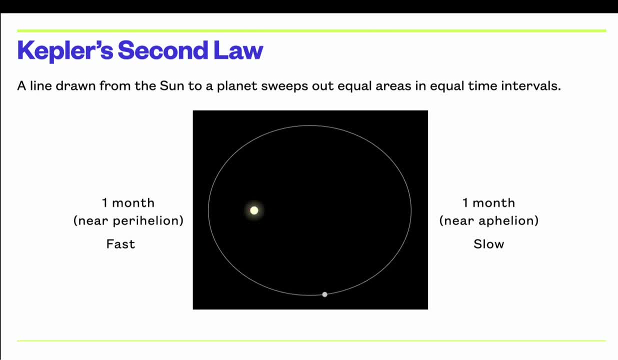 here's a little animation. So there's our planet. it's swinging out. it's going slower out there, now faster and closer. And so Kepler's second law shows exactly how the planet speeds up as it falls in closer to the Sun, and then slows down as it. 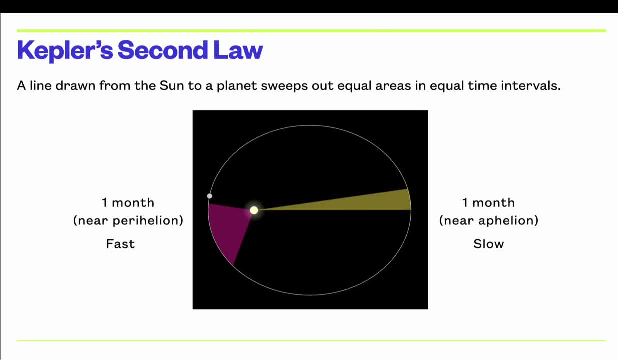 pulls farther away. As we'll see in the next lecture, this is actually the same as saying that angular momentum of the planet is conserved, So we'll prove that this is just a direct consequence of conservation of angular momentum. Finally, Kepler's third. 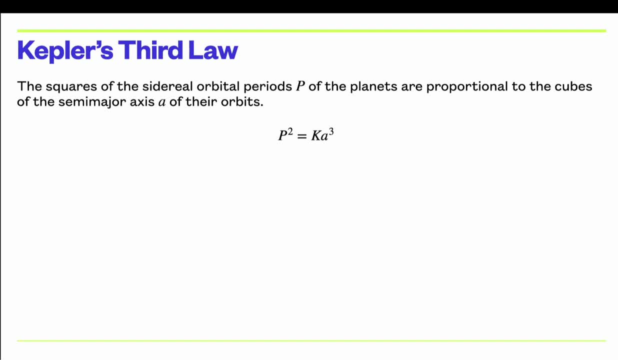 law relates the periods and semi-major axes of different planets in the solar system. So it says that the squares of the orbital periods p of the planets are proportional to the cubes of the semi-major axis of the orbits. So just that p squared is proportional to a cubed. 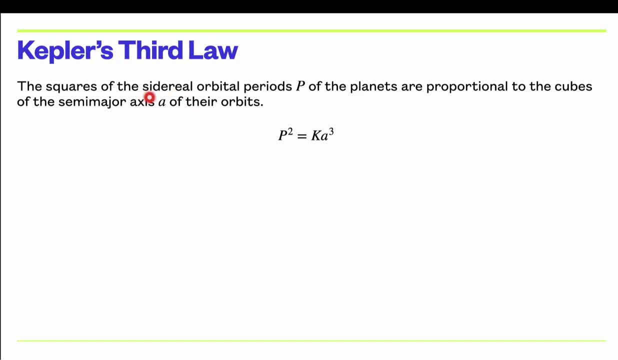 Sidereal, remember that just means measured in an inertial reference frame, not relative to a rotating reference frame. So again, p is going to be the period which we'll measure in years. a is a semi-major axis measured in astronomical units, and k is just defined as 1 year squared per astronomical. 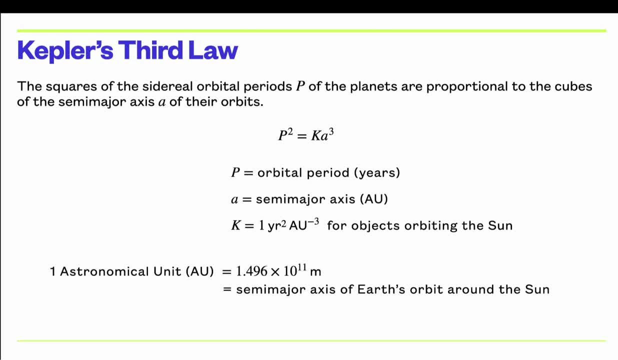 unit cubed, So you can just think of k as equal to 1 if p and a have these units. And again, an astronomical unit is the semi-major axis. So we have a semi-major axis of the Earth's orbit around the Sun. that works out to about: 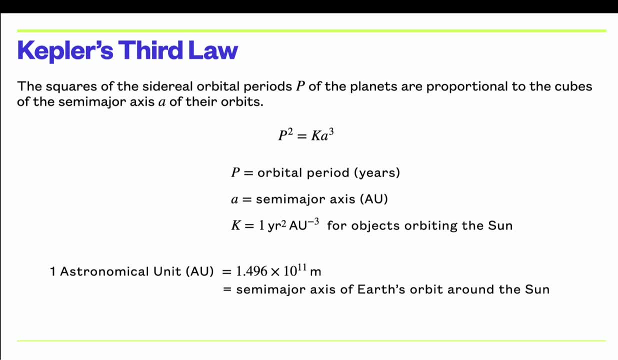 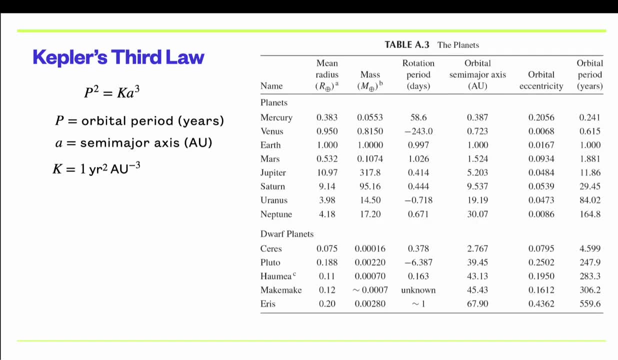 150 million kilometers, or 1.496 times 10, to the 11th meters. So let's go back and look at the table in the back of your book. It also lists over here. the well it lists. there's the semi-major axis that we talked. 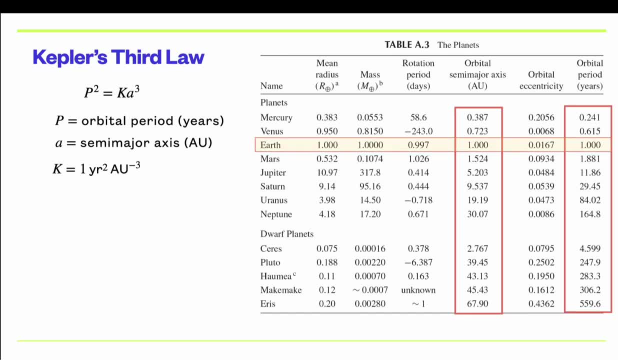 about before, and it also lists the orbital period. So let's look at the Earth. By definition, the semi-major axis is just 1 AU and it's also has a period of 1 year by definition. So here this is trivially satisfied. p squared is 1, a squared is 1, 1 equals 1.. 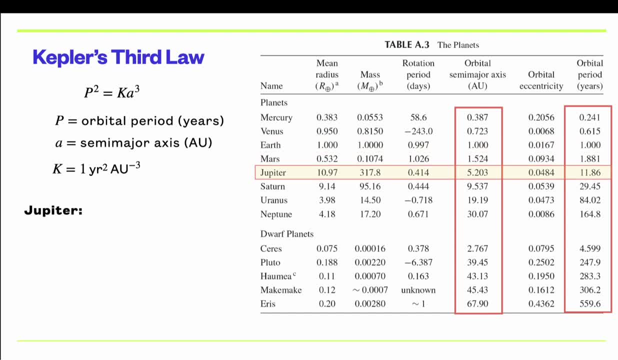 So Kepler's third law holds: Let's try a different planet, Let's try Jupiter. So the period is 1 AU. 1 AU- 11.86.. So if we square that you get 140.7.. The semi-major axis is 5.2 AU. 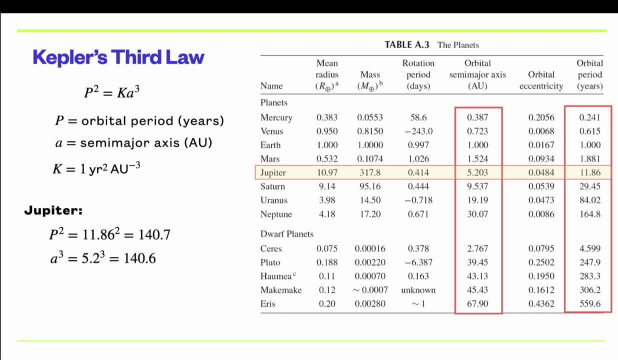 You cube that number, you get 140.6.. So within the errors, the significant figures of the data that we're given, these are in agreement. So this kind of just this example just shows that Kepler's third law at least works for. 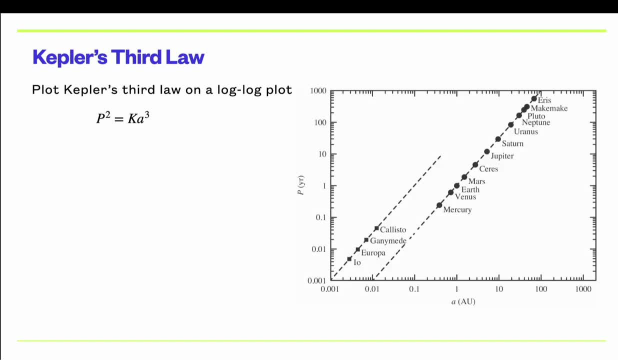 Jupiter. It's interesting: if you take the data in the previous table and then plot it on a log-log plot, you get this nice result that all of the planets line up on the line. So here's Kepler's third law that says that p squared is this constant k times a-cubed. 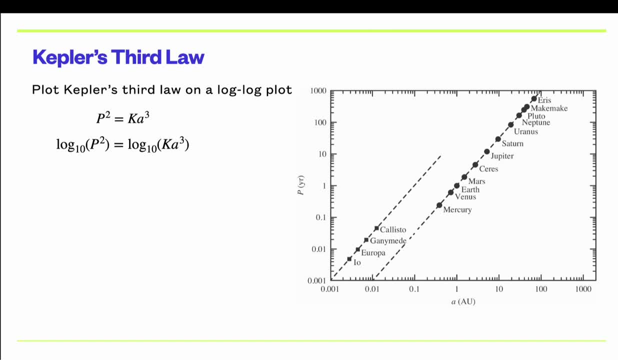 We're gonna. if we want to plot it on a log-log plot, we're gonna take the logarithm of the planets, collegheatcom log of each side of this equation. so if you take the log of p, squared, and then the log of k, a cubed. 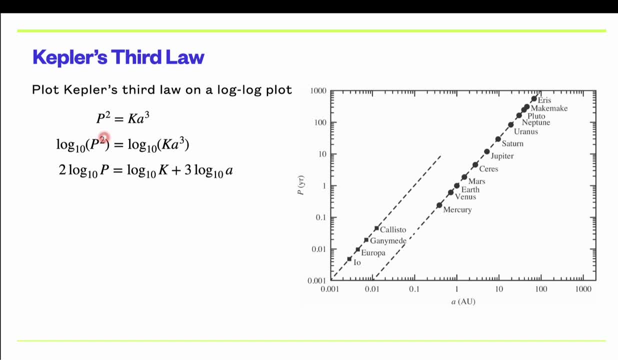 we can remember- you can pull out the exponent here- that that p squared the the two up here comes out in front. uh, when you take the log of the product of k times a cubed that you separate them out like that. so you have the log of that constant k plus 3 log a. and now, if you just divide through 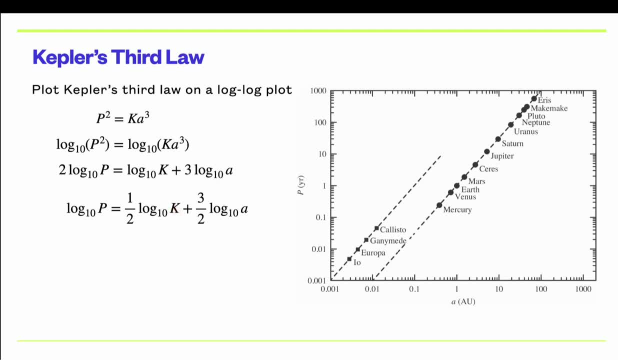 by the two, you get that the log of the period is one half log of k plus three halves log of a. so now, if we plot this on a log log plot, basically what it means is that instead of plotting the period on the vertical axis, we're going to plot the log of 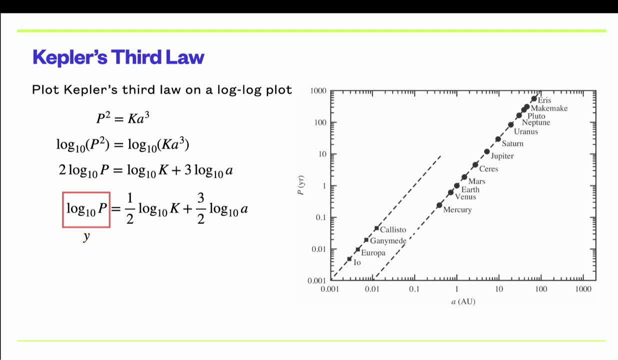 the period. so this will be what we're plotting on the y-axis, on the y-axis, on the x-axis, we're plotting the log of the semi-major axis a and we can see that there's a linear relationship now between y and x. so this constant here is just an overall y offset. so that's just a vertical shift. and then the slope. 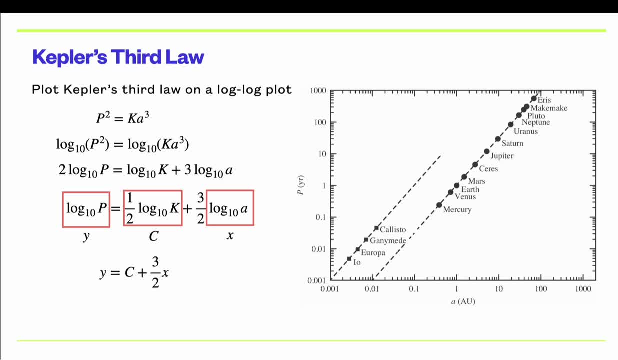 of the line is just going to be three halves, so you can write this expression as: y is equal to a constant plus three halves x. so this is just the equation of a line. this is a general result. so if, whenever you have a power law, meaning if you have one thing is equal to another variable, to some power, and you plot a power log, 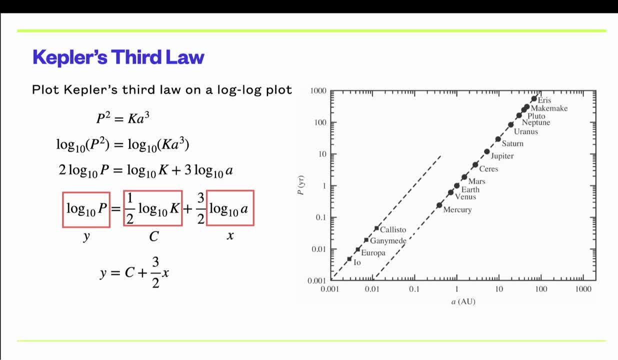 a power law on a log log plot, it always comes out as a straight line. there are tons of power laws in astronomy which we'll see, and so this is a good trick and we'll use this many times in this course. so the reason that this is useful is that you can take all the data. 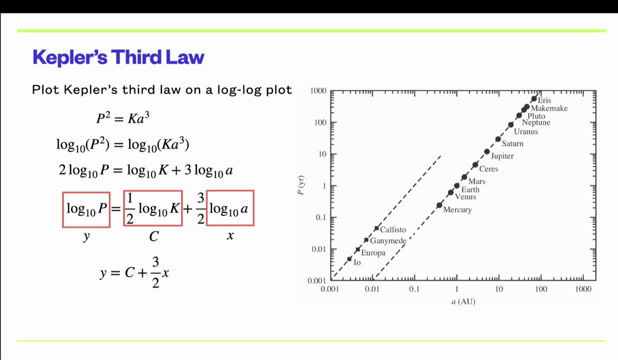 you can plot the periods and the semi-major axes of all the planets and you, if you see that they line up in a line like that, you know that there's a power law relationship between their periods and semi-major axes. and by by, if you look, if you can measure the slope of this line. 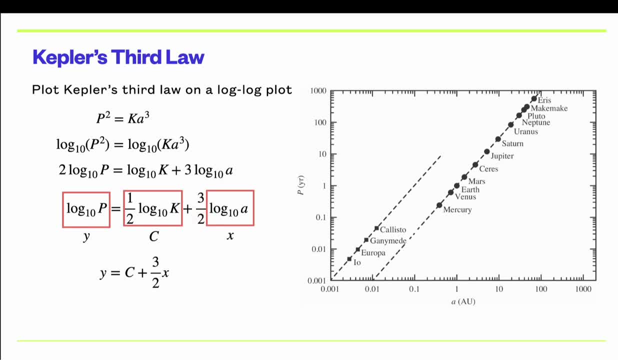 that would give you this, um you, this would give you what that power law relationship is. so, basically, the fact that that's a three ash power: it means that the period goes as the semi-major axis to the three abs power. this constant- here we'll see in the next lecture- depends on the mass of the object that the planets are orbiting around. 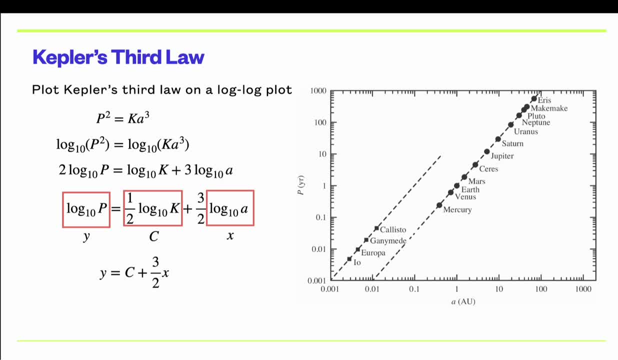 so if you look at uh period and semi-major axis data for the moons of jupiter: uh, here are for the moons of Jupiter plotted. they also follow a power law relationship with the same slope, but you see that they they fall on a different line. that's been.